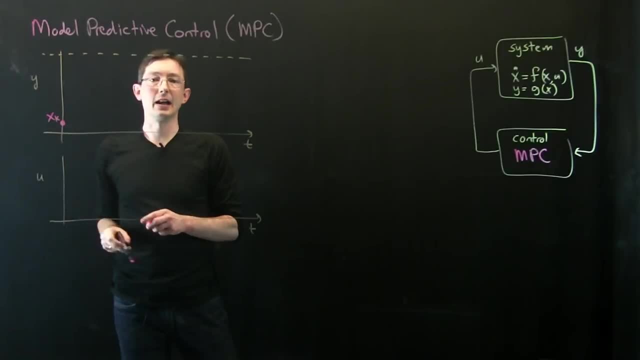 let's say that I have the whole state x and this is at time k, So x at k. And let's say y equals x, just to make this easier, Then what I'll do is I will start my system, I'll initialize it at time: k, xk. 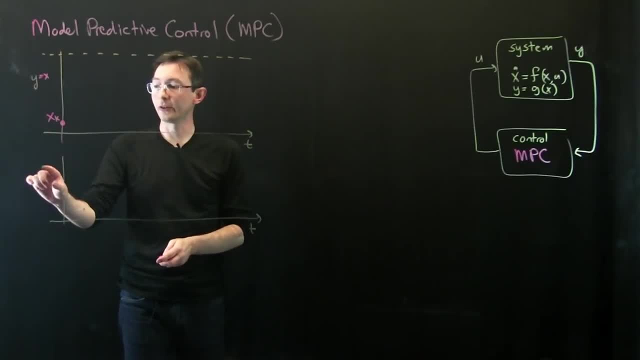 And then I'll run an optimization procedure over the inputs to try to find what is the best U over some short window that gets me closer to my desired objective. Okay, So there will be some window of time. Let's call this my horizon. 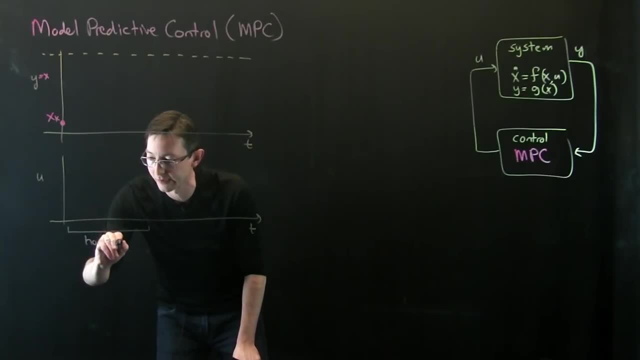 That's what we call this in MPC. So I've got some time horizon And what I'm going to do is I'm going to optimize U over that time horizon. Okay, And maybe what that looks like is some kind of strategy like this: 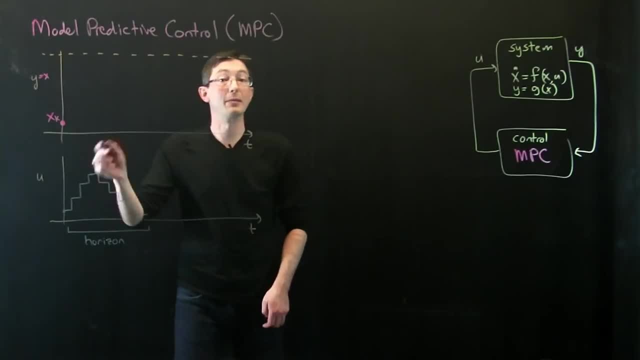 Maybe I'm just making something up, Maybe that's the U that comes out of the optimization procedure that I run here. Then what I do is I essentially just lock in the first value of that optimizing control law And I see where my system goes. 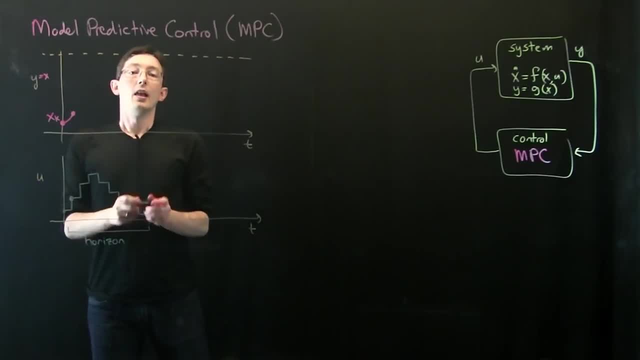 So now my system maybe goes there. Then what I do is I shift my horizon over 1 delta t and I re-optimize. So now, maybe the system didn't go exactly where I thought. So instead of doing this now, I think that my optimal control should be. 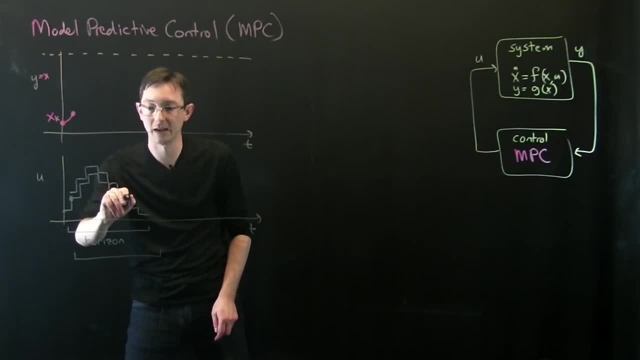 a little bit more aggressive, something like this: I'm just making this up again. Okay, And so then what you do is you essentially pick that next optimizing control, lock that in and see where your system goes, And so over time, 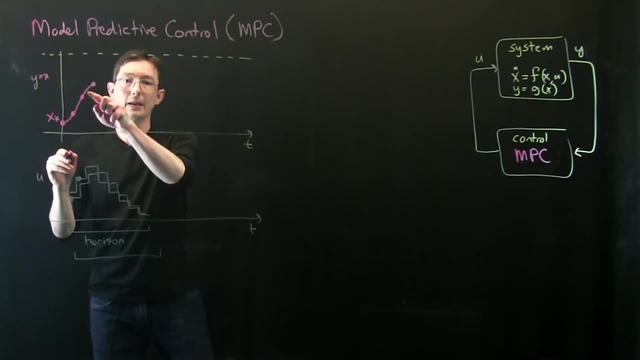 you can essentially watch your system step forward And at every new time step you reassess what the optimal optimizing control input U should be over some kind of moving horizon, And you only enact that next instant control law, that next step of control. 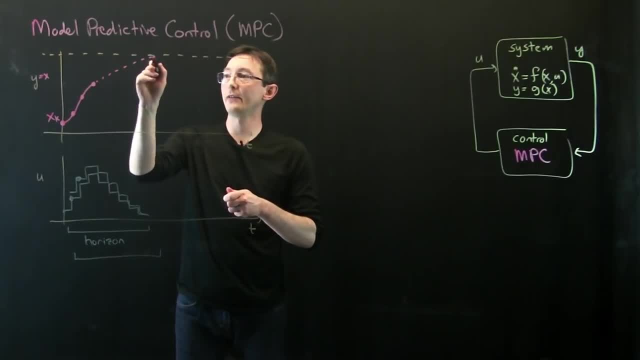 and see where your system goes, And you can essentially get very, very, very good control, even for strongly nonlinear systems. that achieve that Okay, That achieve your desired objective, Okay. So if I write this control down, you would actually say that my control k. 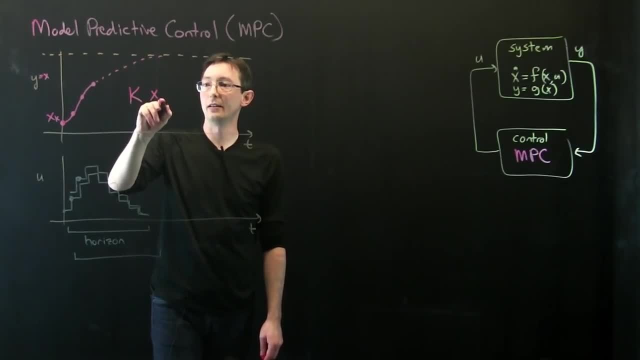 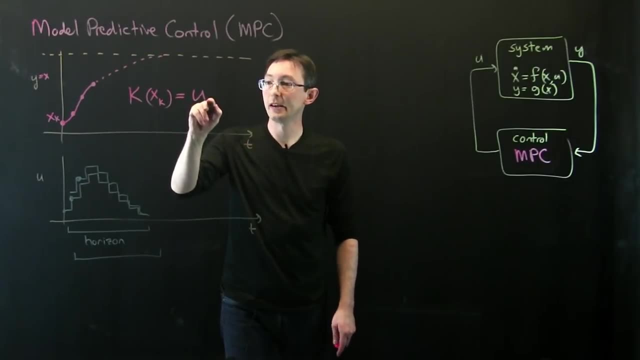 my control signal k at time, little xk would be. whatever my optimal control U is at time step k plus 1 based on time step k. Okay, So I'm going to decode this for you because I found this a little confusing. I found this a little confusing the first time. 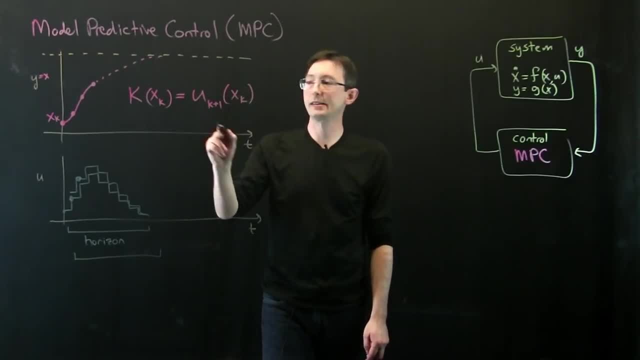 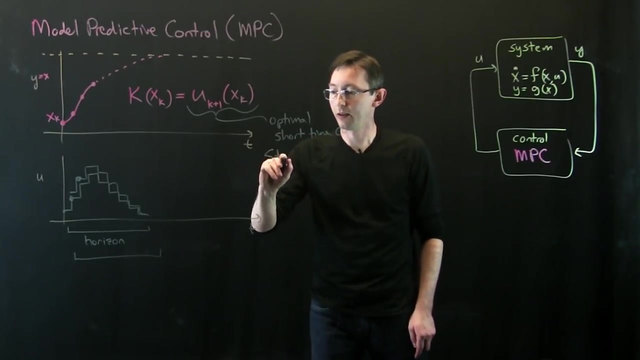 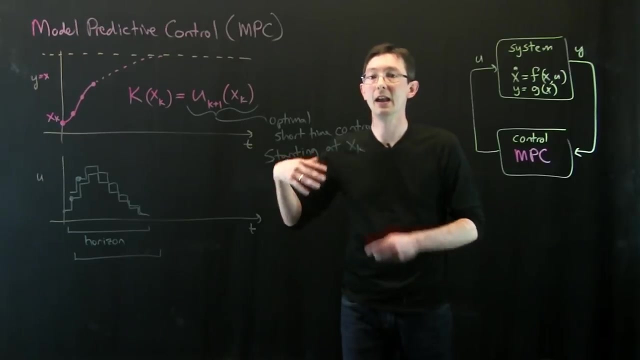 So U k plus 1 of xk basically means this is my optimal short time control strategy: short time control starting at xk. Okay, So I initialize this optimization at xk. I figure out this long trajectory of U's that would optimize my objective function. 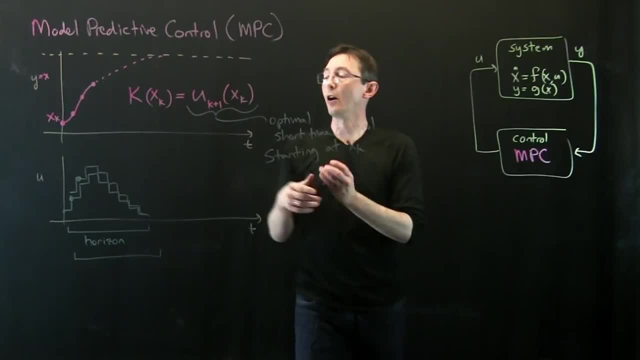 starting at that initial condition given this model, And then I only implement the first time step. This is the first time step. So I run a simulation and I optimize my control over many time steps, but I only implement the first time step. That's my control law at time k. 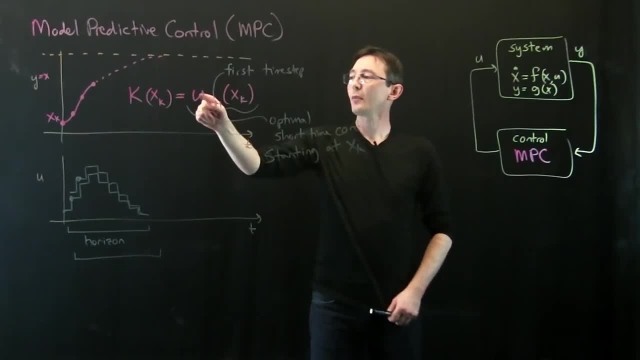 Then my x moves to xk plus 1. I reoptimize an entire new control trajectory starting at xk plus 1. And again I implement the first time step of that new optimized control strategy. It steps me forward, and so on and so forth. 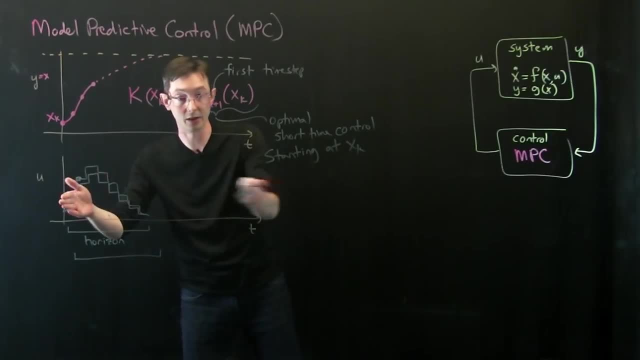 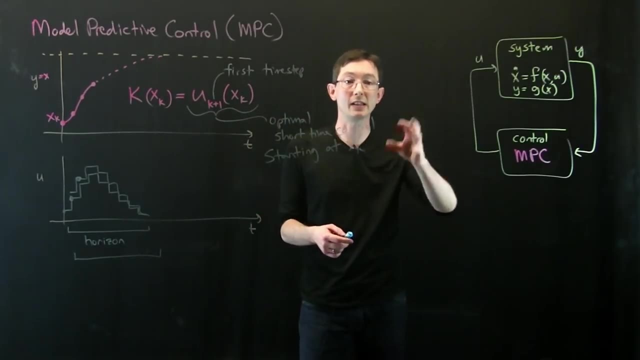 So every time step, I'm rerunning this entire optimization forward in time over some short time window to see what is the best possible U given my new state and what the dynamics actually did. Okay, So that's the basic idea of model predictive control. 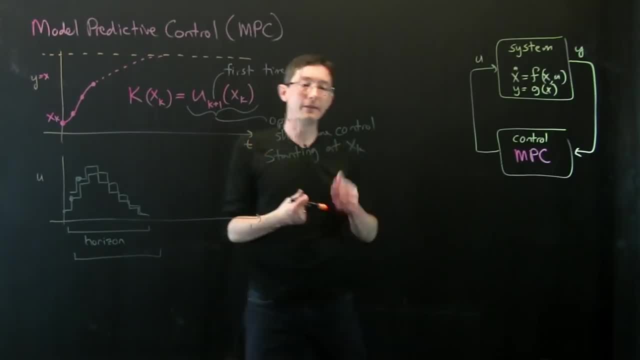 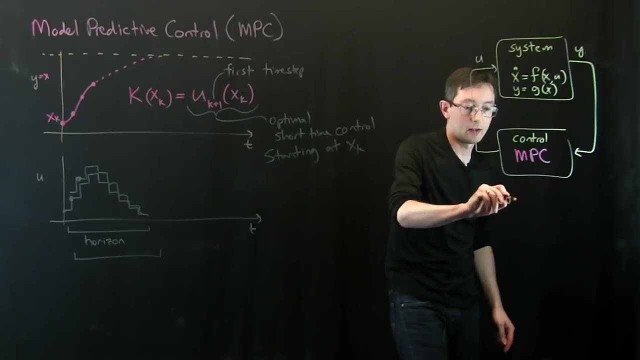 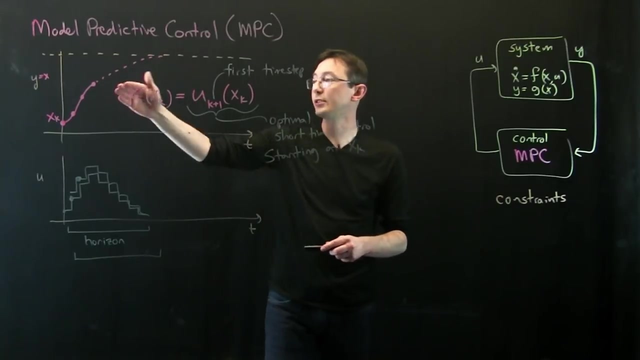 Now why is this so powerful? I think this is so powerful for a number of reasons. One is that you can impose constraints, So I can have constraints on the state of my system. So, basically, I can do a control so that I never hit some boundary. 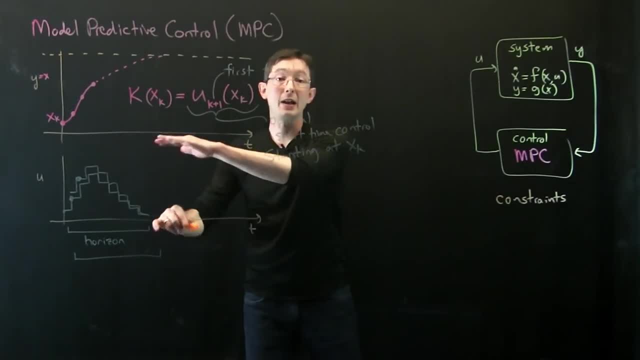 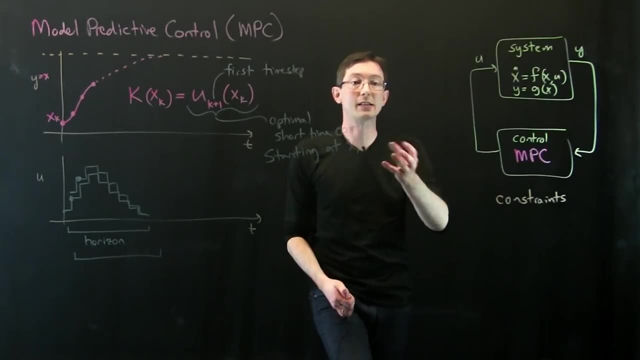 so I stay within some bounds, But I can also constrain my input, which is very, very important. So in a lot of control strategies that we've seen up until now, the actuation is this kind of control is a continuous variable And oftentimes your controller. 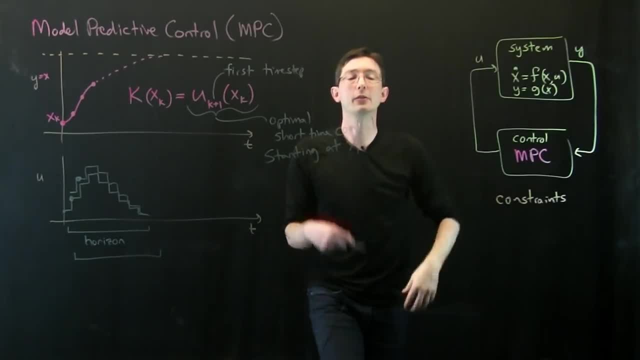 would make unrealistic demands on what you could do. So, for example, if I'm designing a cruise controller, if I design my control law badly, then it might command U's which are unphysical. It might say: go a million miles an hour. 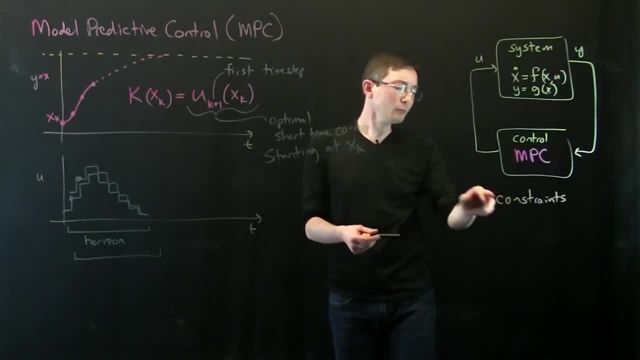 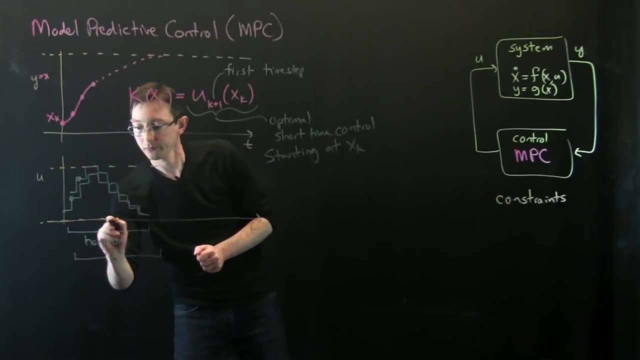 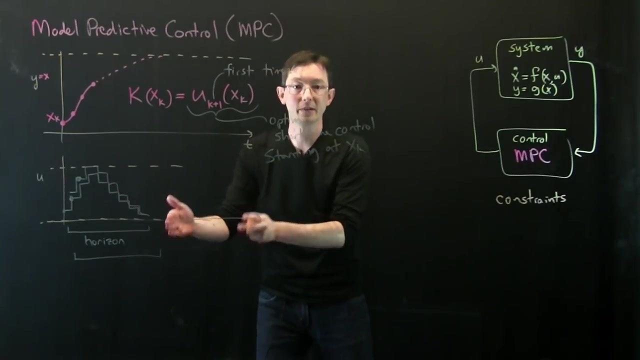 for a fraction of a second and then slow down. What model predictive control can do is it can essentially put bounds on what your control signal can actually do. So when it's running this optimization loop for every time step, when this optimization is running, 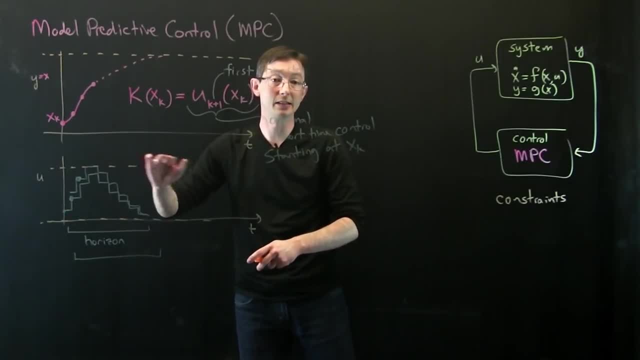 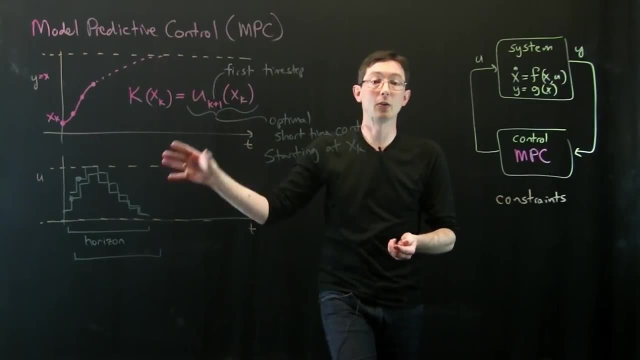 it can essentially constrain the optimization to not hit these max or min values. So that's really cool. It can run these hard constraints or soft constraints on the state or on the input. It works for nonlinear systems And there's a few ways you can think about this. 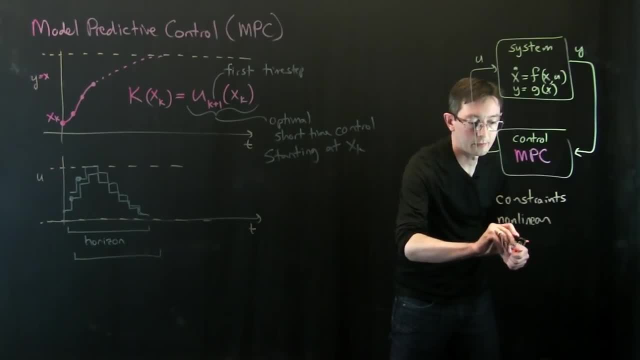 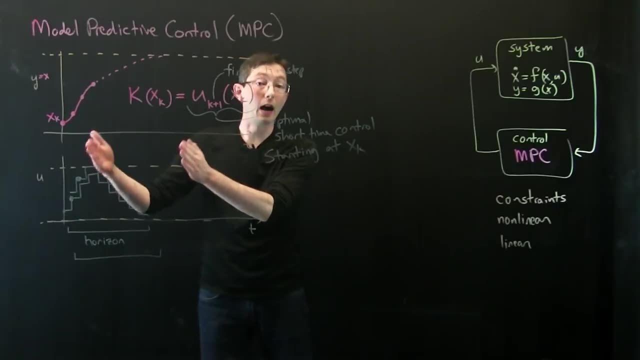 So let's imagine that I had a linear system But there were some disturbances or noise or something like that. So I can determine the optimal control signal for a linear system using something like linear quadratic regulator And I could use that for my MPC short time optimization. 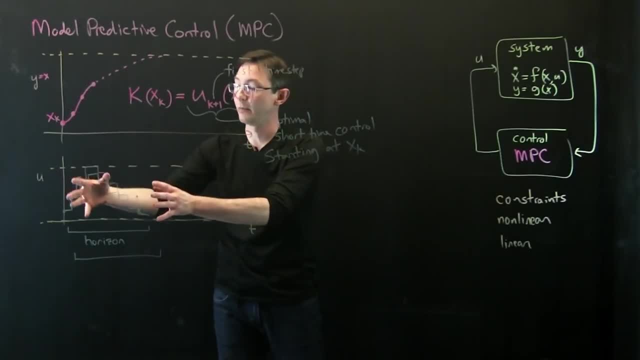 And then if there's some disturbance or some changing parameters in my system, those will compensate over time. If I have a nonlinear system, what I could do is I could take my nonlinear model and I could linearize it about that particular state, And then I could do. 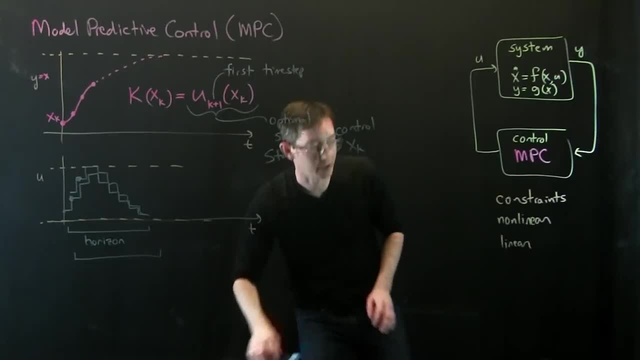 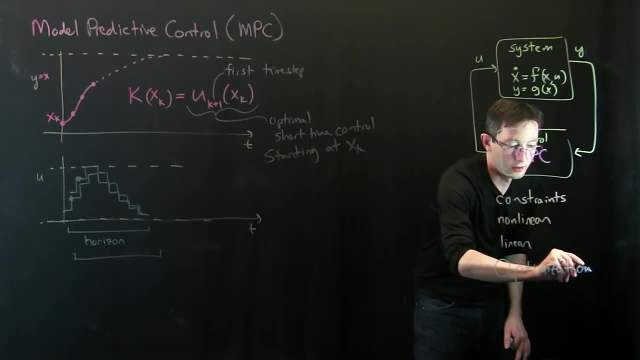 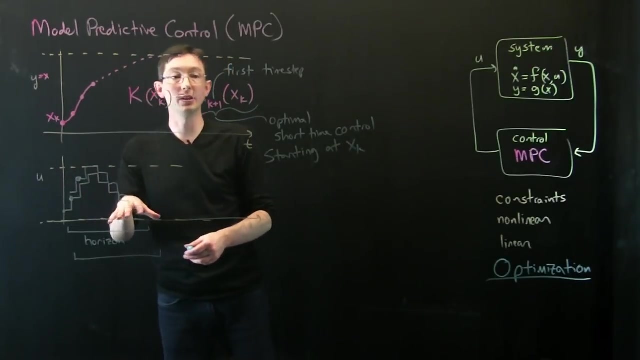 kind of linear optimization. So maybe what I'm trying to get at here is that optimization is the heart of MPC. MPC is built around an optimization Every single time step. I'm re-optimizing this control strategy U and then just picking the first time step. 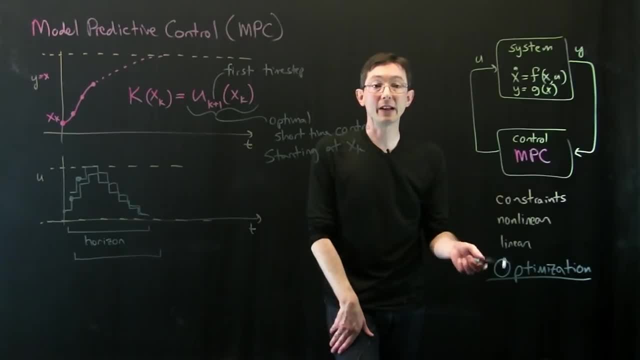 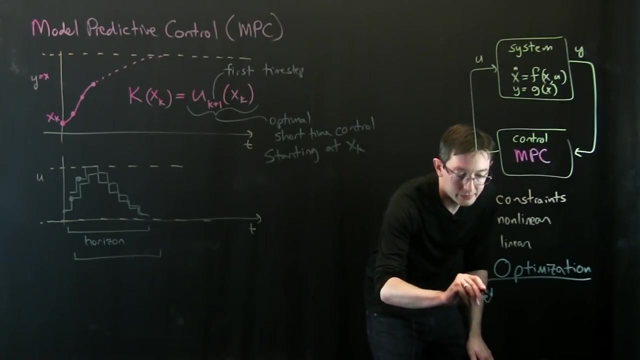 and re-initializing and starting over. So this is a little bit expensive because I'm running this full optimization at every time step And this is enabled by increasingly fast computers and fast hardware. So this essentially relies on fast hardware to be able to run this optimization loop. 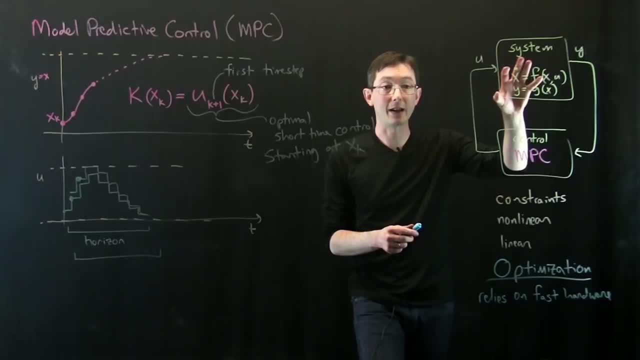 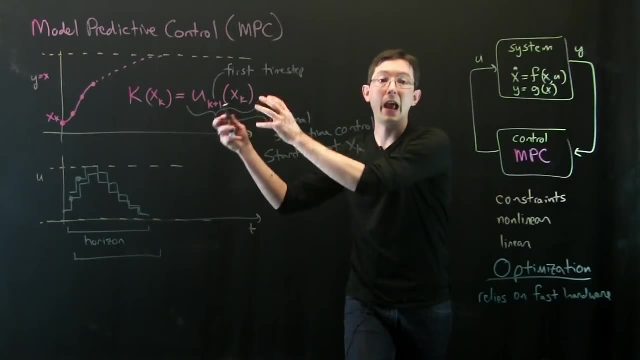 instead of usually, if I do something like a linear quadratic regulator or a common filter, I run my optimization offline on a you know a big computer and then I take those results and I hard code them on my fast online control system. MPC is different. 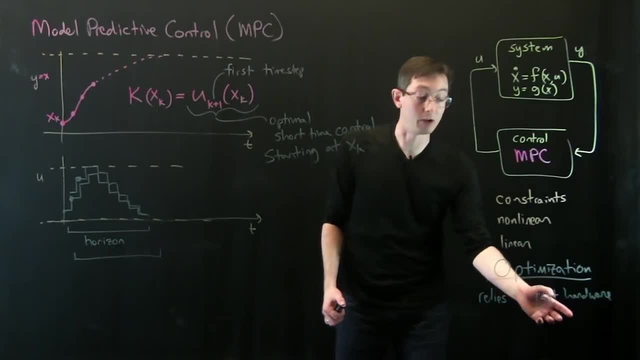 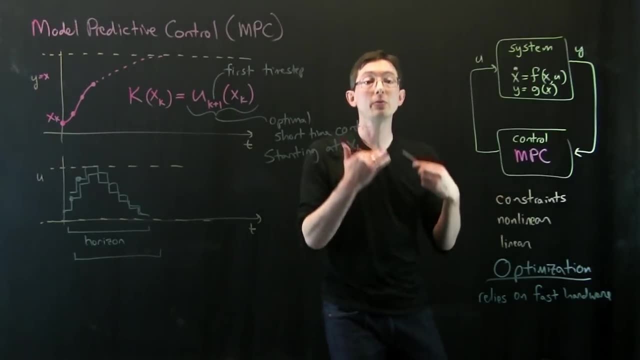 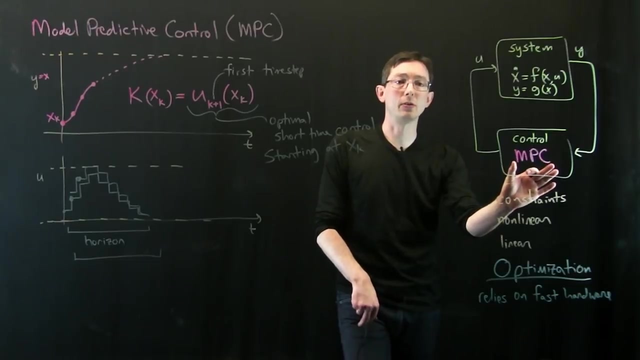 It relies on the fact that you have fast computational hardware to run this optimization online at every time step. Okay, Now we know that there are known optimal solutions for U for linear systems, So oftentimes model predictive control will be applied to linearized equations of motion. 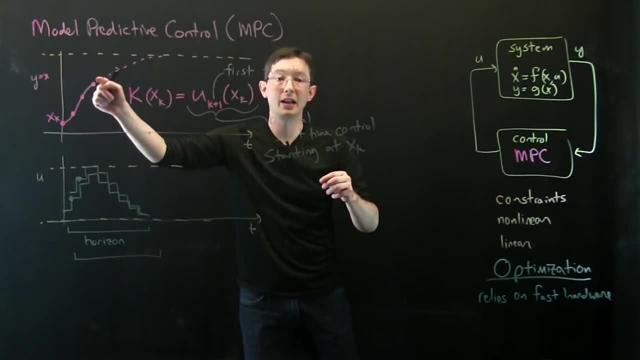 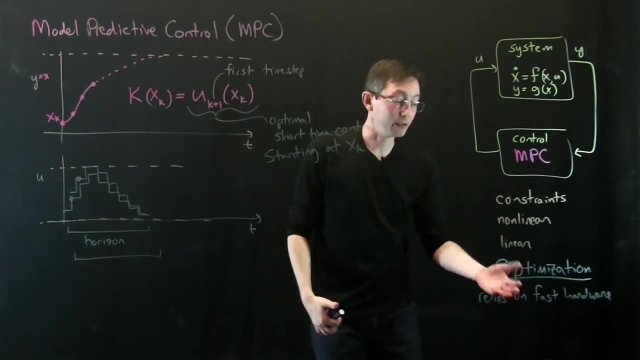 Even if I have a non-linear system, maybe I'll compute the linearized dynamics at every point x and I'll feed that into a linear optimization, because that's fast. But increasingly, now that computers are getting faster and faster and faster, it's becoming increasingly possible. 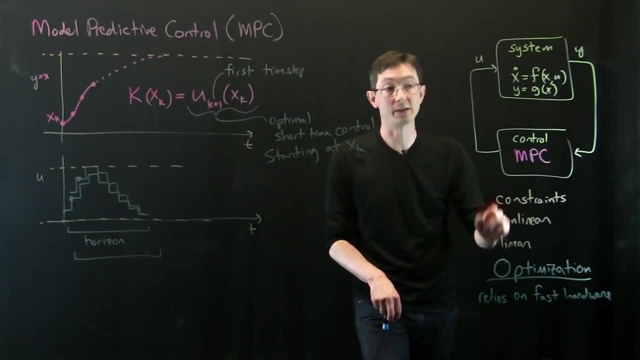 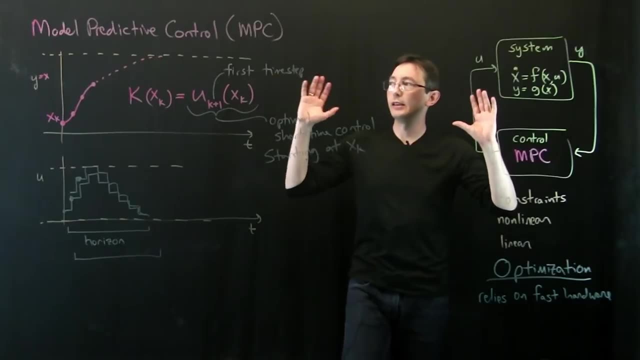 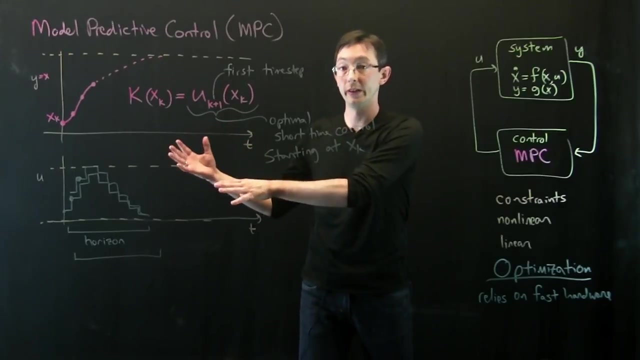 to actually directly optimize the non-linear equations of motion, if you have them, Okay. So kind of the big picture here is that now, instead of doing our control optimization one time offline, like we used to do with linear quadratic regulators, we can do this optimization. 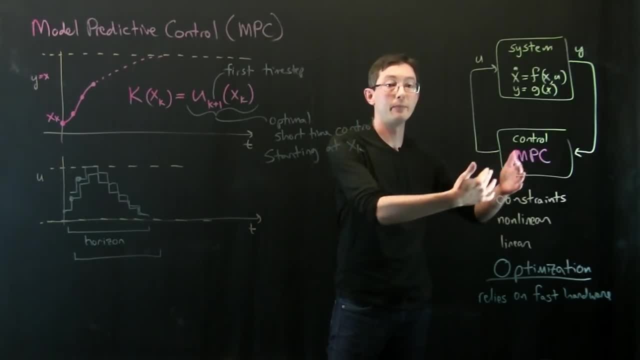 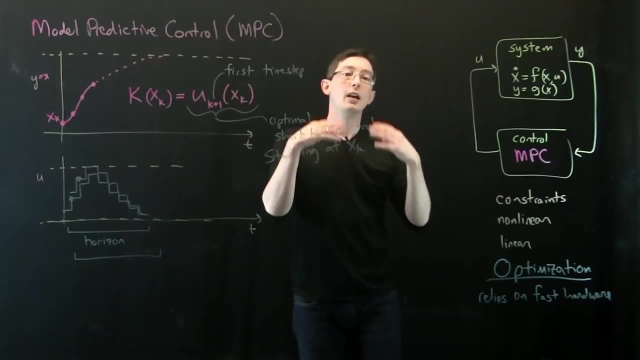 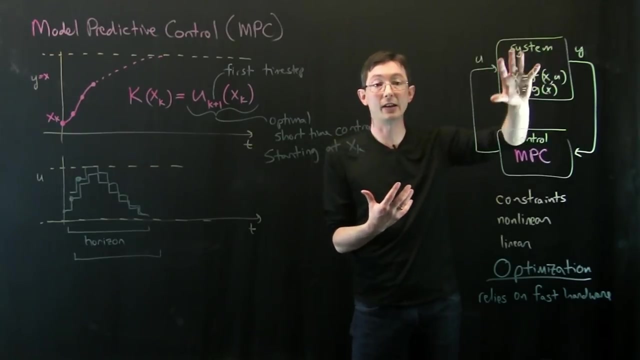 continuously at every time step of our system, and we can modify our control behavior if our system starts to deviate or if the dynamics start to change. Now this has driven a tremendous amount of interest in system identification, because this relies on having a system model. 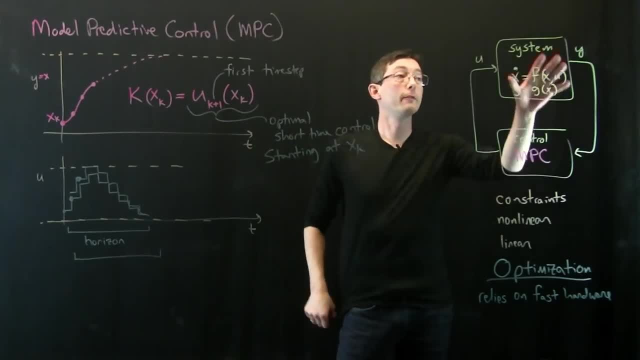 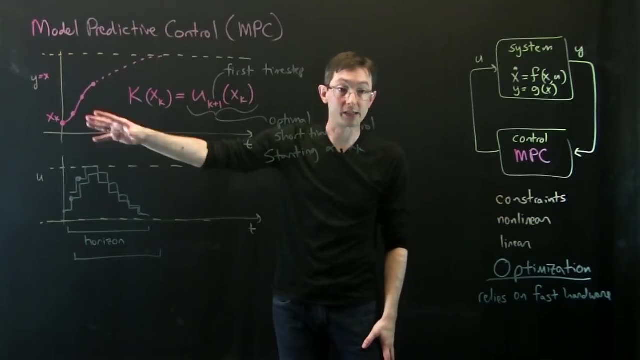 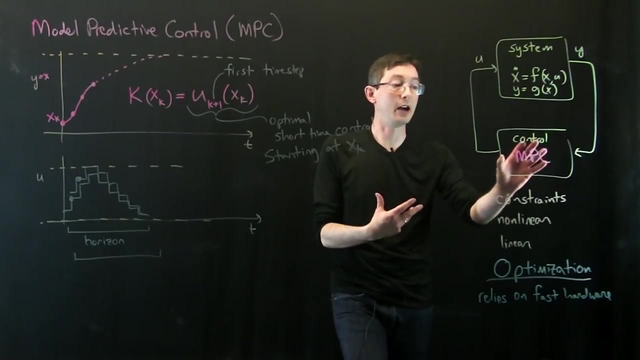 So because of the power of model predictive control, we're very, very interested in getting good system models that we can actually use. So non-linear and linear models of our system that we can control. Linear is the easiest and fastest to optimize. So a lot of model predictive controls. 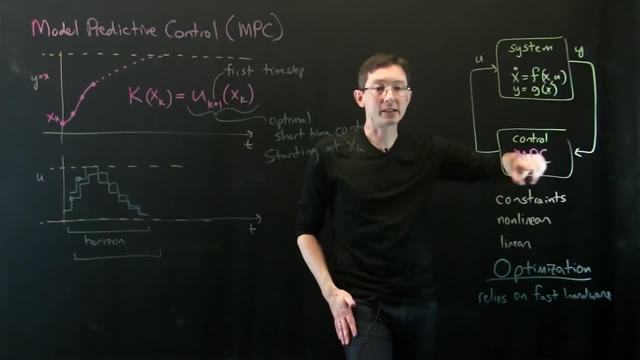 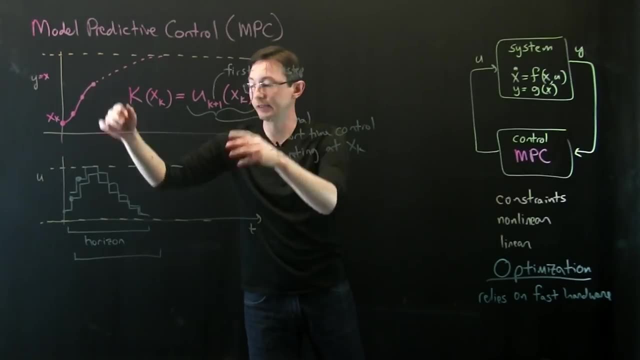 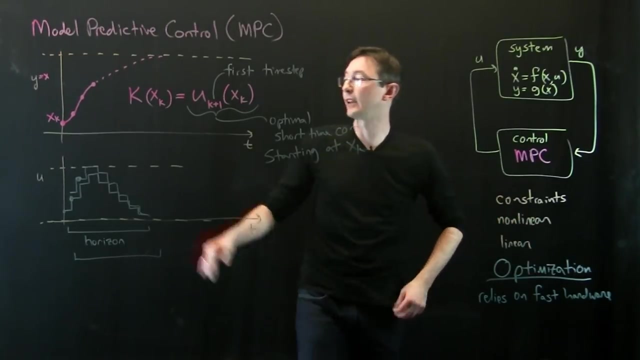 are wrapped around linear models And of course there's this feedback. So if my system doesn't do what my model says, then I just reinitialize and make a new prediction. So model predictive control is more flexible than traditional linear control methods because if the system starts, 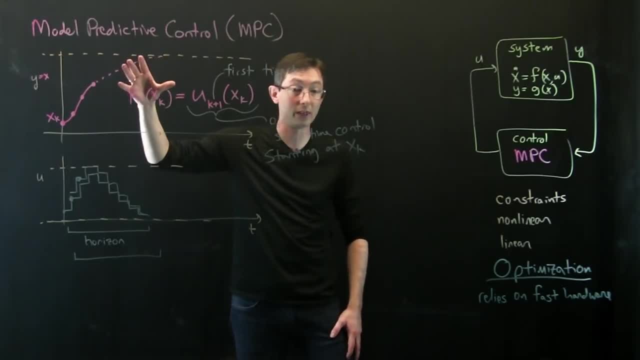 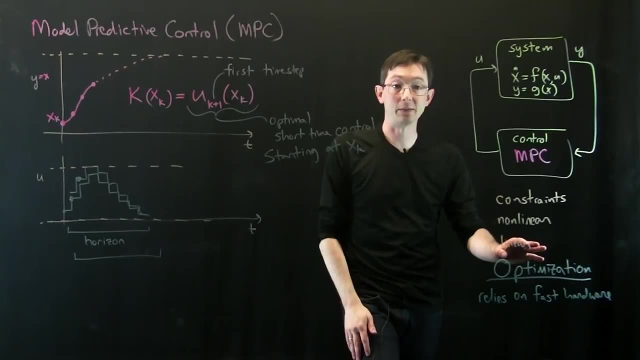 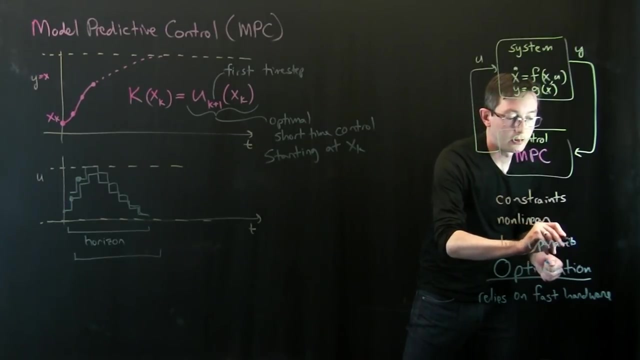 to move or deviate or doesn't do what you think it should. you reinitialize your optimization at every new time step Okay. so that's really important is that this is more flexible. Sometimes what people do is linear parameter varying. So essentially what I do,